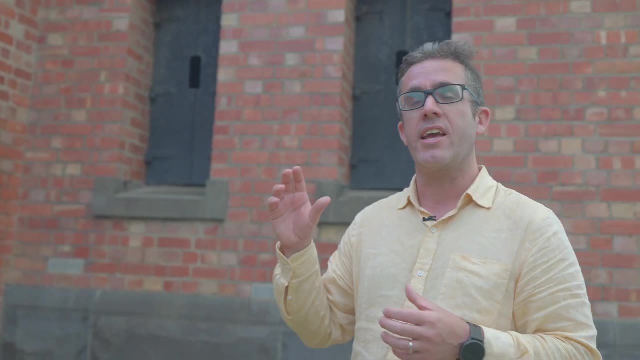 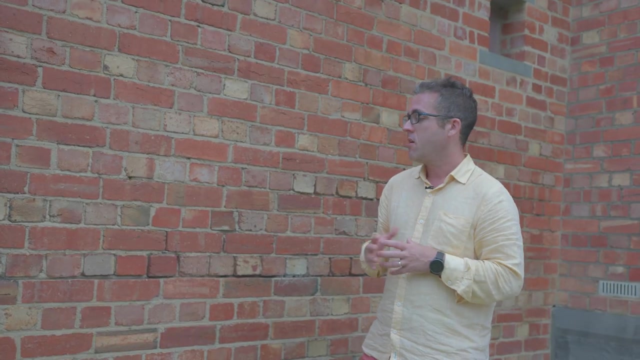 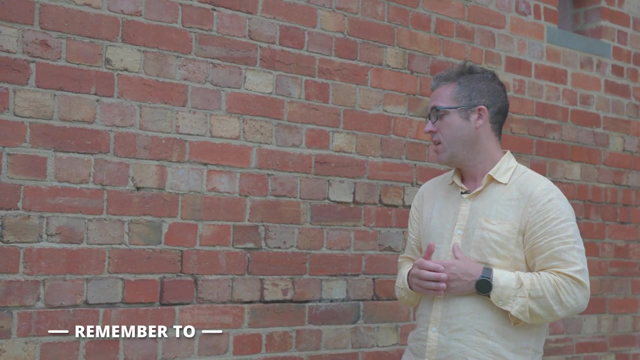 And Queenscliff has this fort that has this amazing brick external facade to it that allows you to understand some of the basics that you need to carefully consider. So, as we can see, masonry structures are built in layers and courses, And the way you lay the bricks will be dependent on what type of structure you're building. 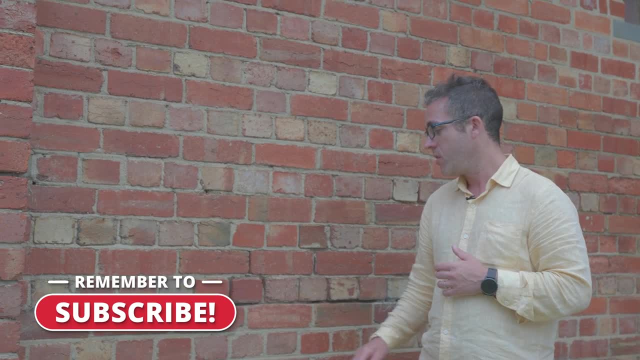 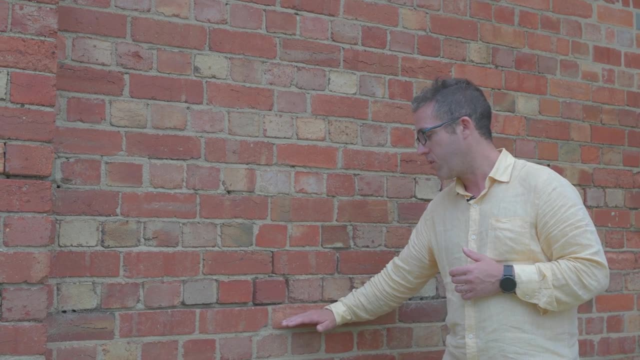 And we can see here at this wall that we've got a number of different courses. So we've got our typical stretcher block that you'll see in most modern builds today and even in historical builds, where you've got your one block here. but typically you'll 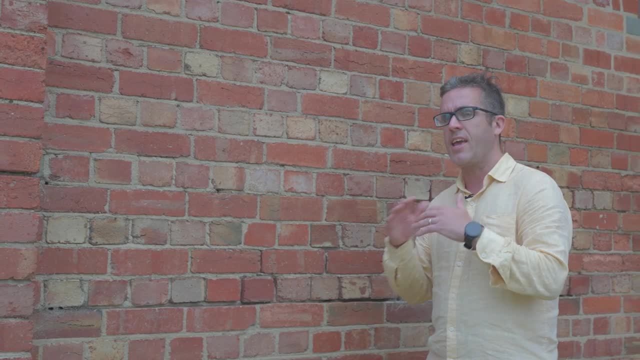 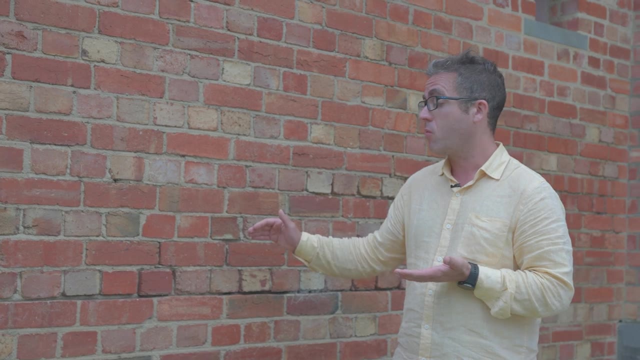 see another block here Overlaying on the joint, So they're keying in. But in this building we can see that we've got our stretcher block and then we've got a header course. What a header course does? it goes into the brick wall, tying one or multiple layers together. 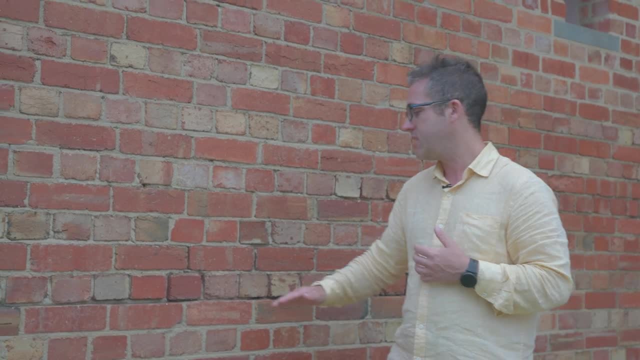 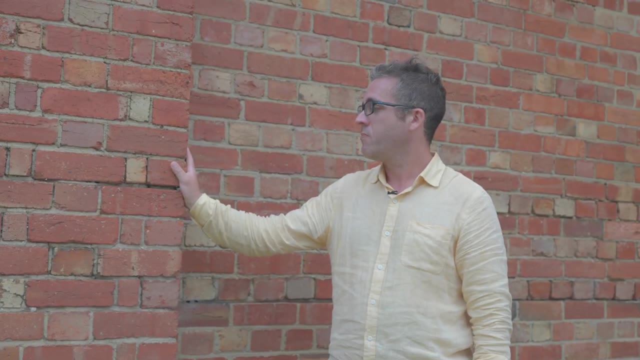 creating a stiffer structure, especially in fences. So we can see we've got our stretcher course, header course, stretcher course and header course. Another key element we can see here is we've got brick piers. So brick piers are typically in walls sometimes if you need to stiffen them up for height. 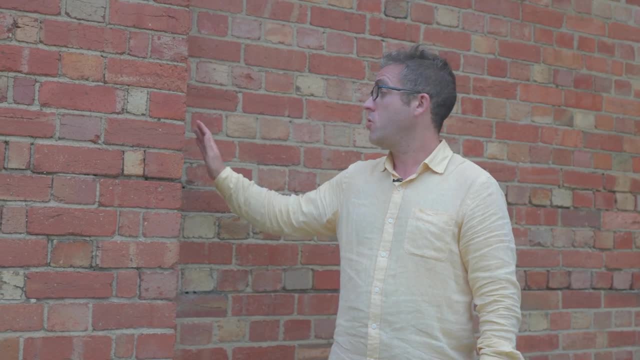 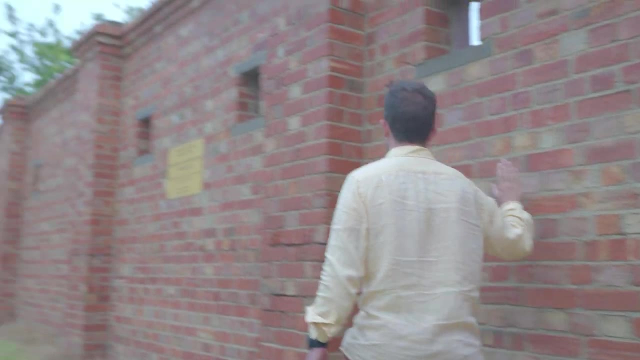 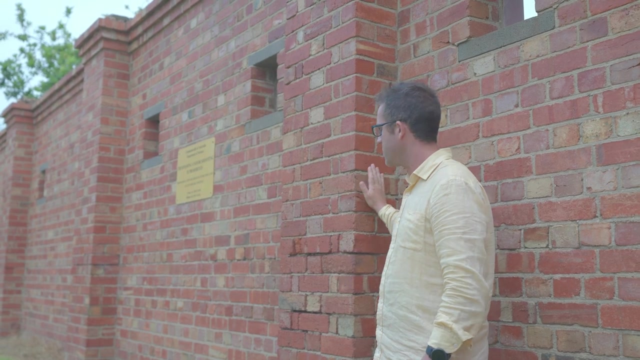 but most commonly done in fences, as it's done here. So the pier is actually bigger. so if we walk across, we can see we've got our traditional fence in between that's thinner, and then we go across to another pier that's essentially bigger. So what allows you to do is create a stiffer structure. 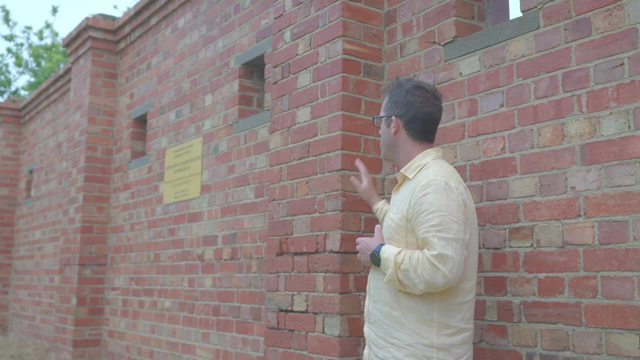 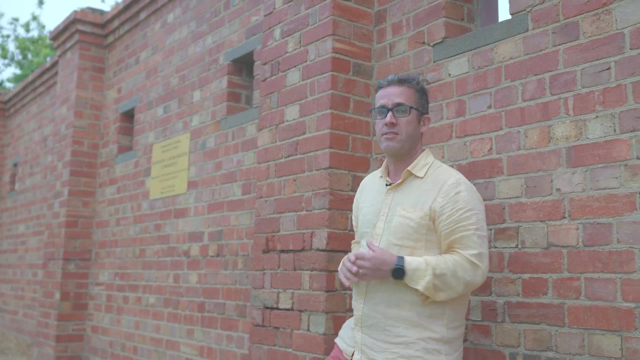 Sometimes you can also reinforce the centers of them. So you'll have your pier, which will be the main spanning element for the height, and you'll have typical wall in between it that will span between the piers. Bricks are also made up of two different types, so you either have articulate, 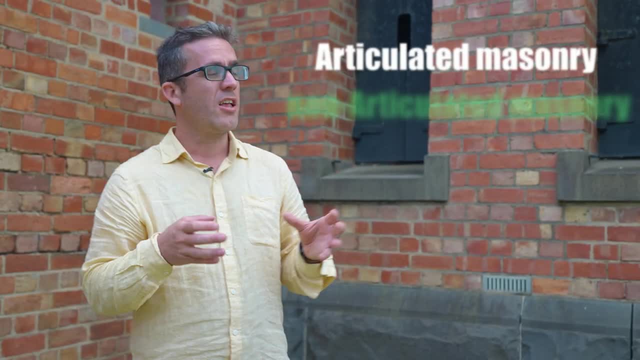 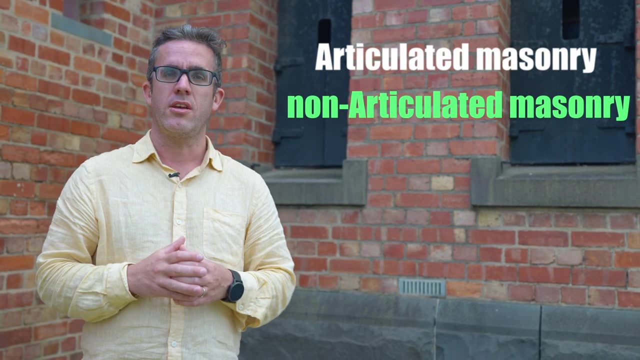 masonry or non-articulated masonry. So articulated masonry is the typical one that you see or have joints at certain centers. There's two reasons potentially why you articulate your masonry versus not. One of the biggest ones is your footing designs, As we can see here on this. 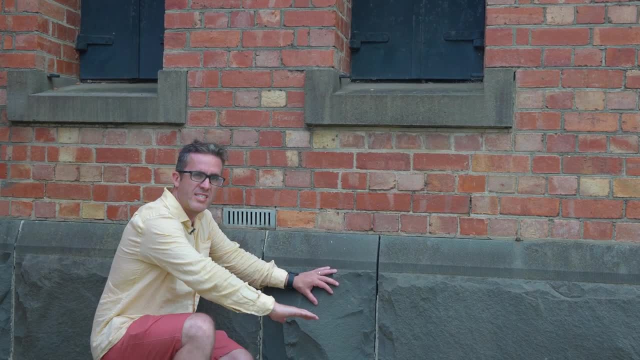 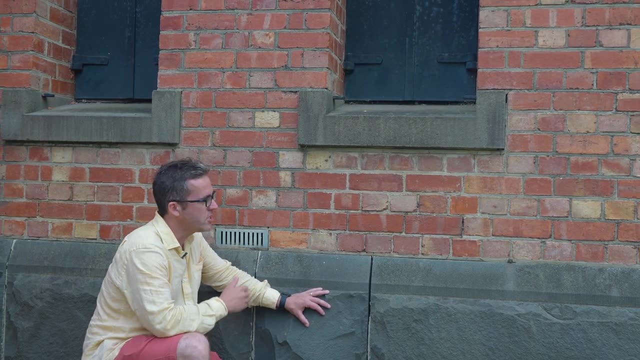 floor. this is a non-articulated masonry structure. So we've got this big footing system here which is made out of bluestone. The reason why they're made out of the bluestone is because of the weight. It's heavy so it won't move very much. They're also bigger, so it helps you span. 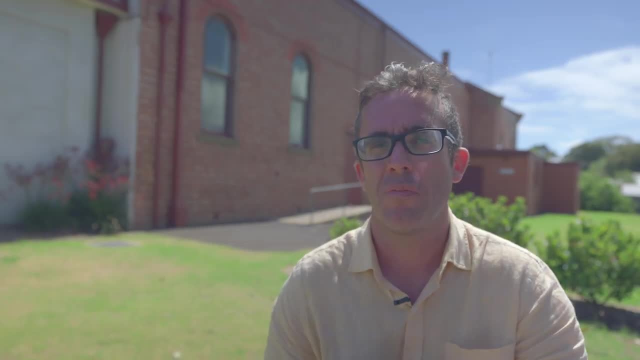 across it. Also, when talking about footings, it's highly dependent on the materials underneath. As we've known from footing designs, soils can be different levels of reactivity, So in a highly reactive soil you're more likely to go for your articulated masonry, as there will be a lot of 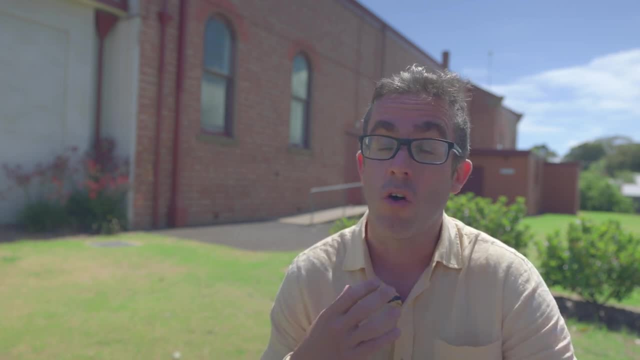 movement, as you'll need a stiffer footing system Where, if you're sitting on rock or sand, you may be more beneficial to go for your non-articulated masonry, as you do not need that stiffer footing design. I'd just like to take a moment to thank the sponsor of this video, Skillshare. Skillshare. 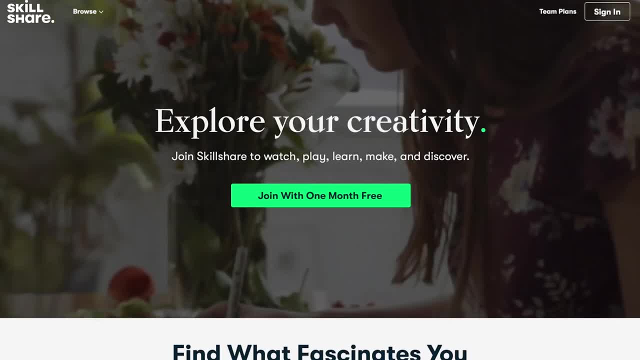 is a place where you can get a free trial of Skillshare. If you're interested in learning more about Skillshare, you can go to the link in the description below. It's a great place where you can invest your time to unwind and relax through the premium content that is ad-free, where you can. 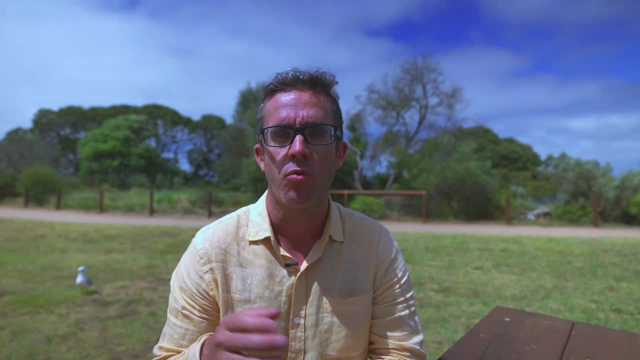 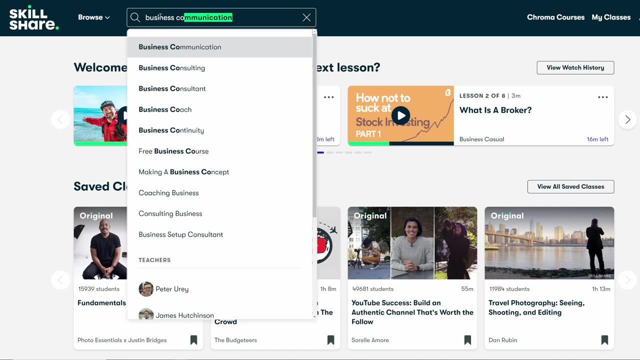 have a variety of courses that you can take to help improve your career. As I've said in earlier videos, your really key assets are improving your communication skills, either that technical, professional, writing or speaking, and they have a variety of courses through Skillshare that allow 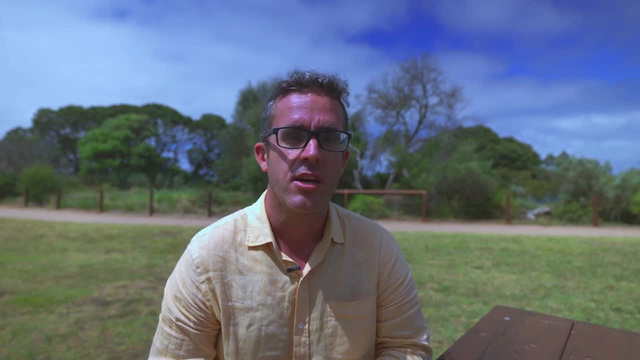 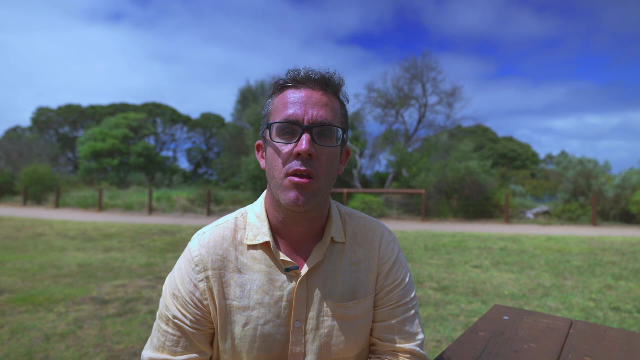 you to improve those. There's also a number of courses on engineering and one specifically on eTabs design. So if you're interested in learning more about eTabs, you can go to the link in the description below. There's a course specifically made in there as well. for you, I also have a link. 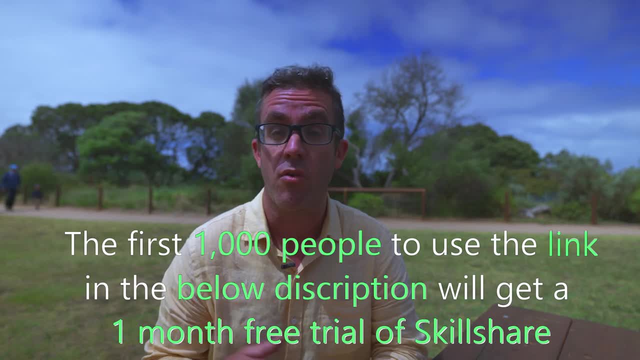 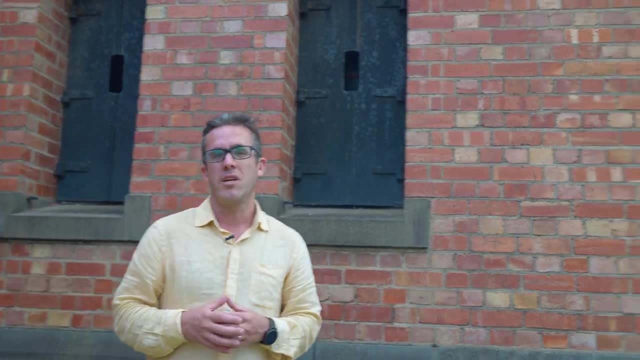 in my below description, where the first 1,000 subscribers will get one month free through Skillshare. So in traditional designs, if you're doing a non-articulated design, your footing system needs to be a lot heavier because it can't allow for that movement. This will also determine. 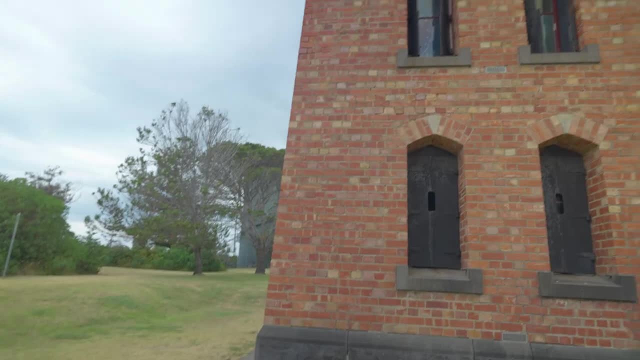 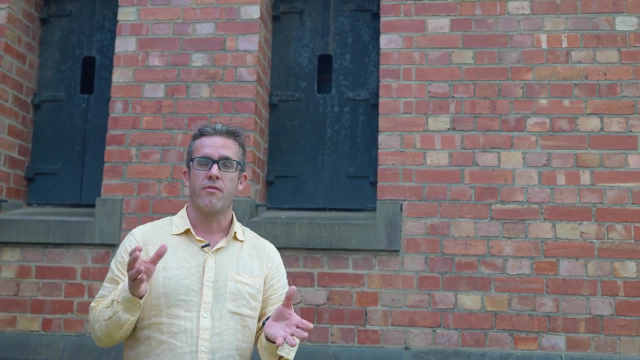 if you've got lintels or headers, You'll need to make sure the lintels are stiffer, as a non-articulated masonry structure only has a limited amount of deflection tolerance that it allows for. Now the reasons why you'd choose one over the other. the first one is that footing system, The 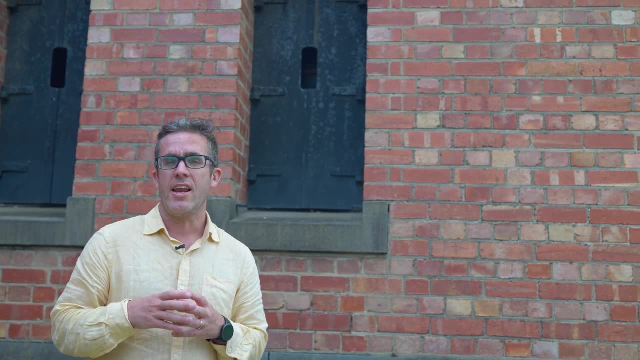 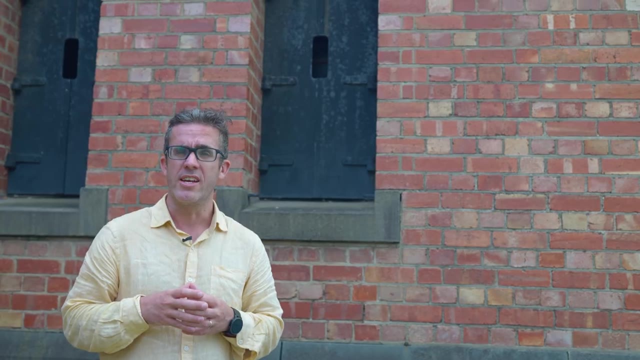 second one is temperature, As a brick wall will expand like any material over a temperature. So we've got a wall that's about 30 meters long with a differential temperature of around 40 degrees. That wall will expand up to 13 millimeters, which is quite a lot of movement that the brick wall 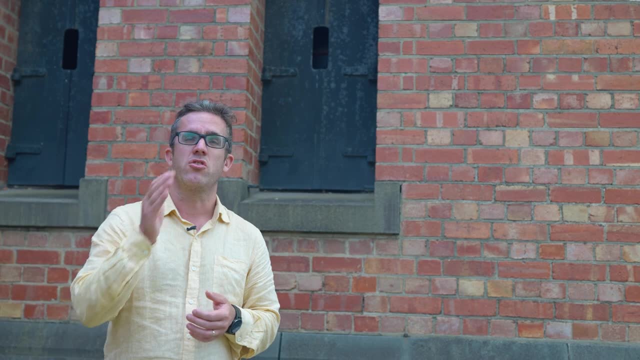 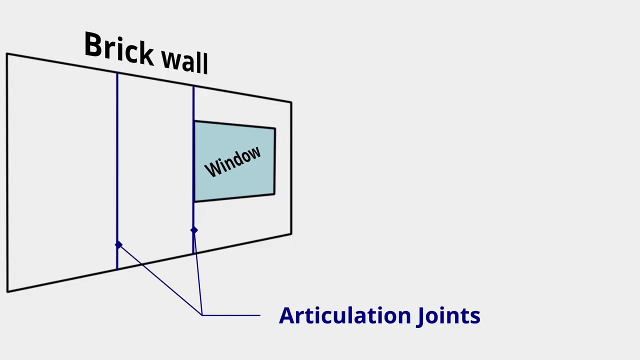 needs to accommodate. So if you've got a really long wall, you will need to make sure you've got articulation joints or allow for some movement, as the wall will potentially crack under those joints. If you've got an articulated masonry, we can see that we've got a lot more articulation. 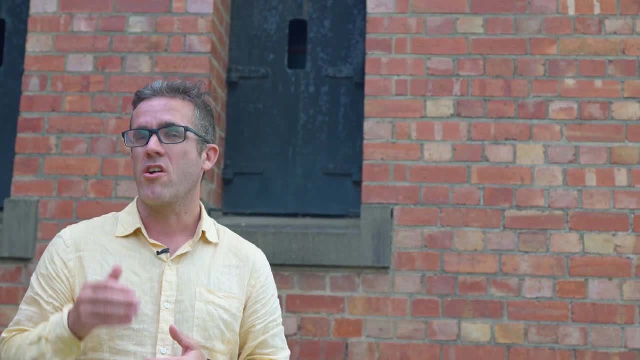 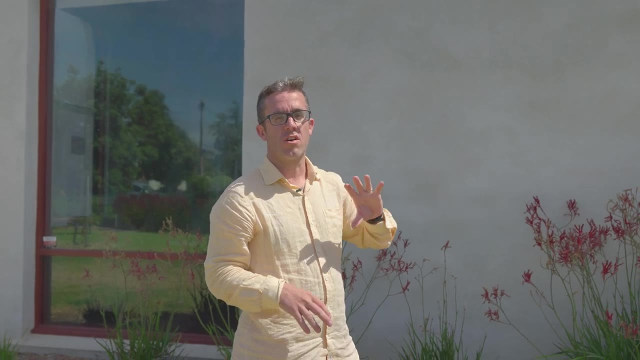 joints. As the footings are moving and the lintels are moving, you need to make sure you're locating your articulation joints in the right locations At this building. here we can see the perfect example between articulated masonry and non-articulated masonry At the start of the 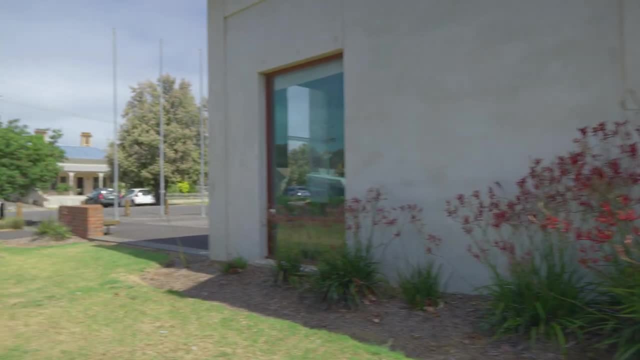 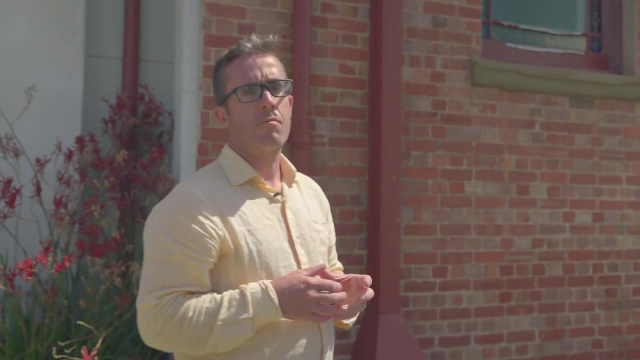 town hall. we've got articulated masonry. We can see this through the beautiful location of these joints above these openings. But if you walk back towards this way, we can see the original building, which is a non-articulated masonry with beautiful arches, And we can see through. 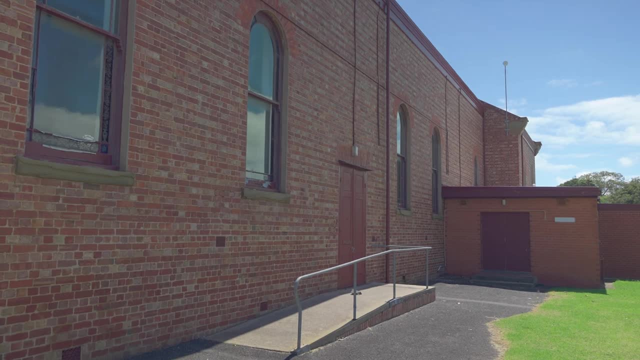 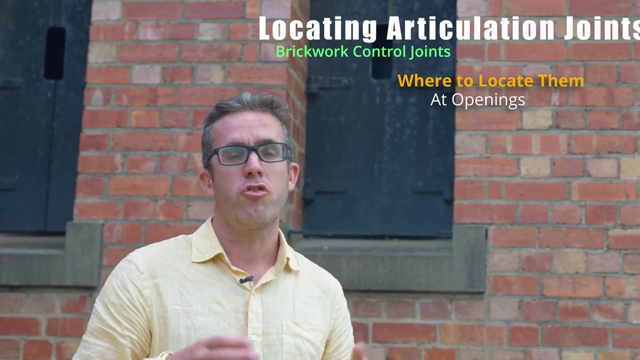 maintaining perfect footings and good detailing. I haven't seen much cracking in the facade of this structure. Typically, you'll need to locate them over either an opening, either on one side or both, depending on how long the opening is. You also need to locate them roughly at about. 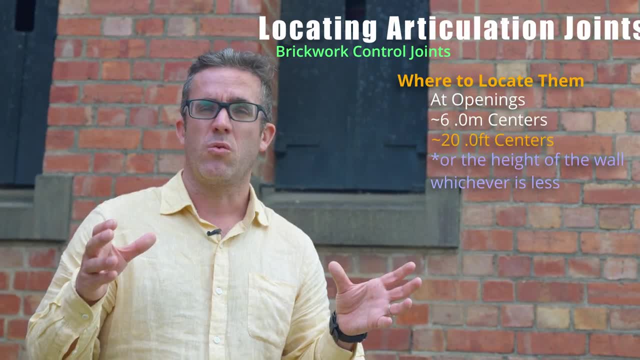 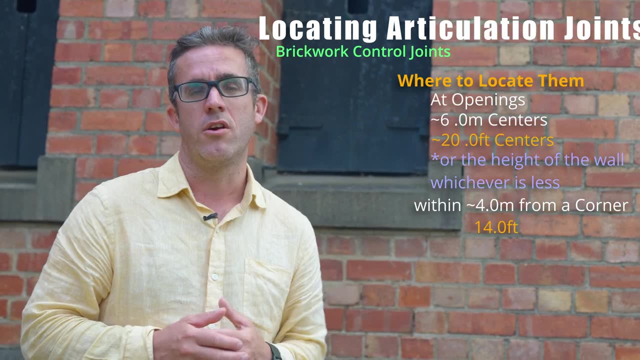 six metre centres, as you need to make sure you're making those grids roughly square, similar to what you would do in concrete, And also corners are really stiff, So you need to make sure you've got your first articulation joint within about four metres of any corner. A couple of key things. 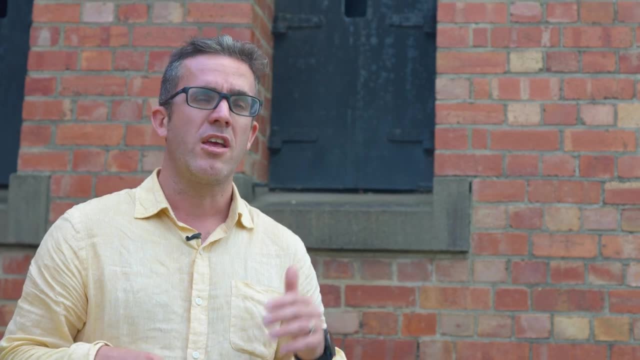 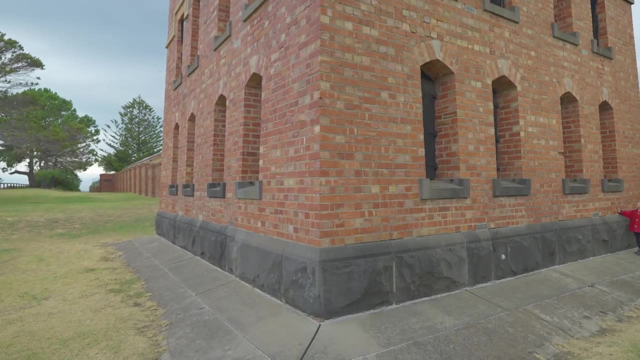 related to masonry design is locating those articulation joints, because they will either be determined whether your structure is going to crack or not. Masonry structures also need to accommodate for lentils and headers. So if we look up here, we've got a couple of arches in here. 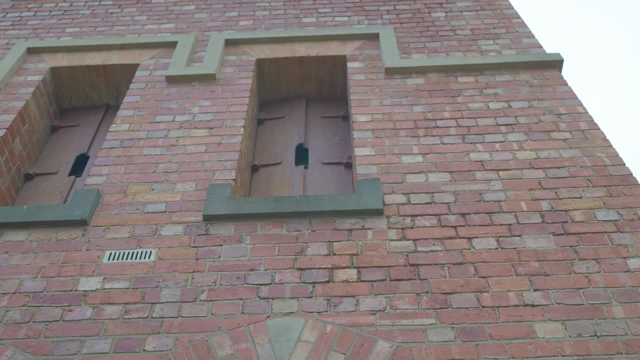 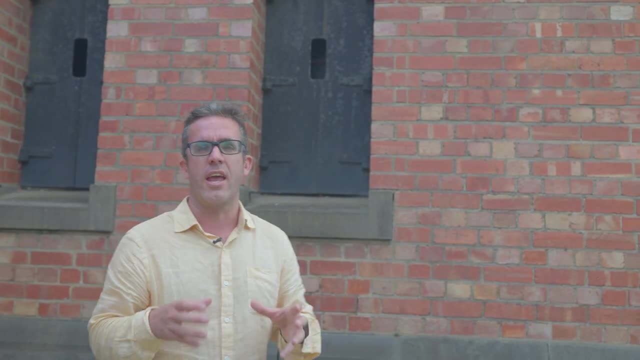 which they're really utilising the benefits of brickwork. See, brickwork, much like concrete, is only really good under compression forces, And the arches that we can see here really emphasise the benefits of this. As the arch we've got here at the lower level, which is 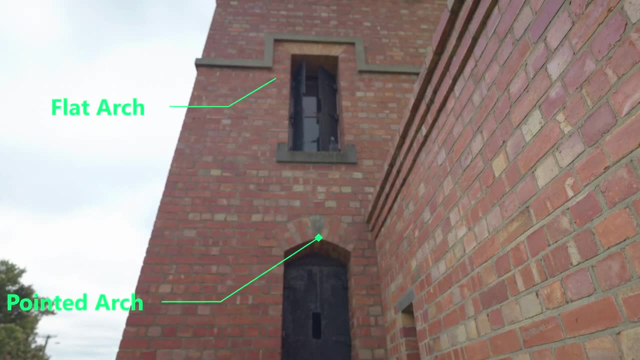 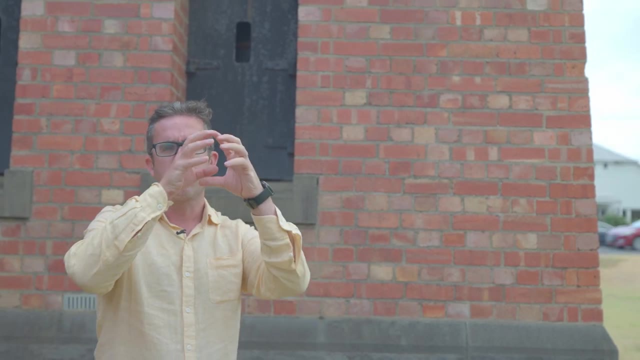 a pointed arch and at the higher level we've got a flat arch And they're both working in the same way. So the pointed arch. it's quite easy to see how that's working, As all the bricks are pitched on a certain level. it's forcing the load down the arches and compressing that location. So 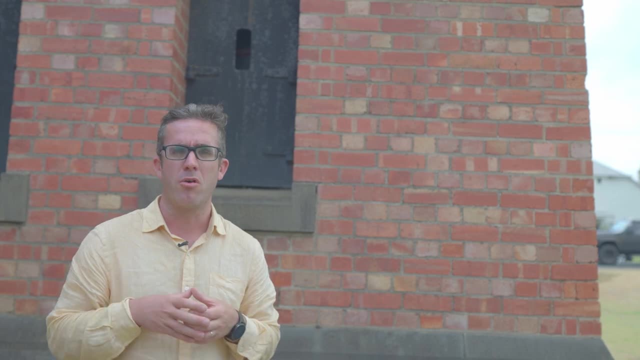 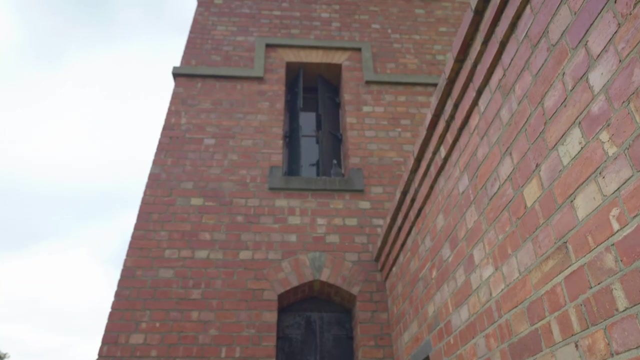 any of the flexural forces or tension forces that would be typically in the bottom of that lentil are overcome by the gravity force. But the flat arch also acts in the same way. As we can see, the bricks are pitched, So as the gravity comes down, it's creating a thrust force at the bottom. So you 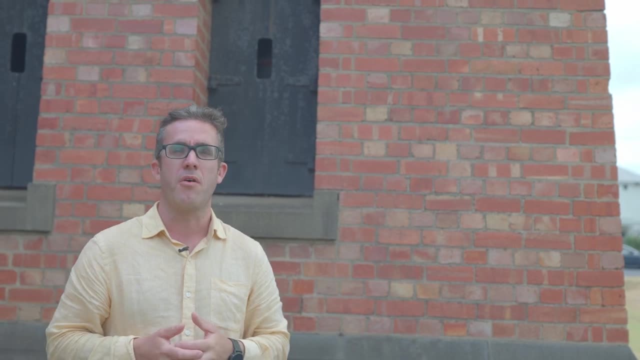 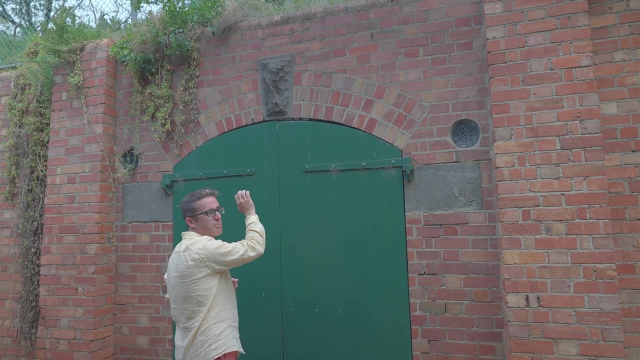 can see whether you've got enough gravity down to overcome any tension forces in the bottom of that arch. So we can see another form of an arch structure here And we can see with our row arch here where it's got a number of different courses and they're essentially built in rows up to the 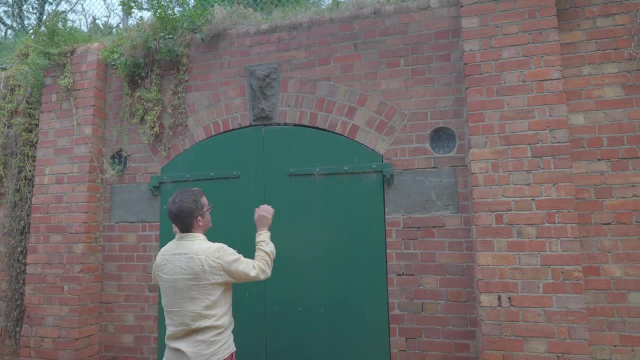 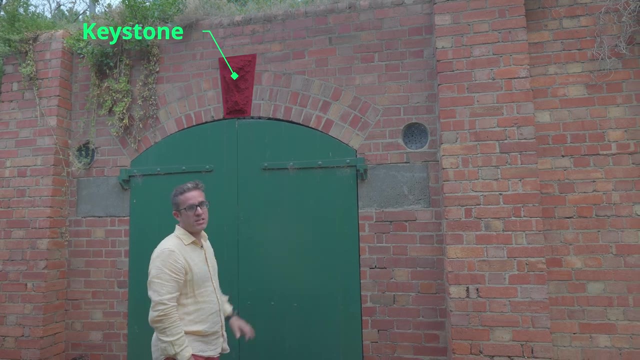 central point, which is the keystone. So to build this, they would potentially have temporary supports underneath here, building up the rows of brickwork over the top and lastly, putting in the keystone. that will lock everything into place. When we look at the structure here, we can see. 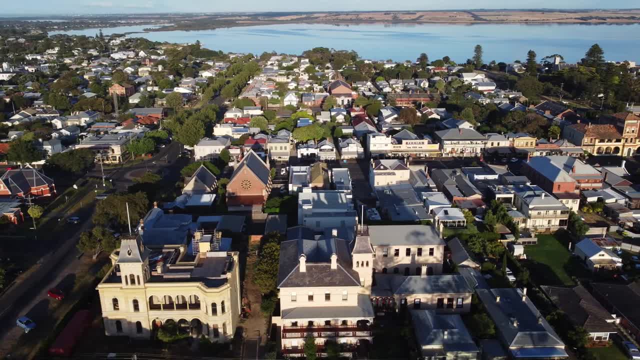 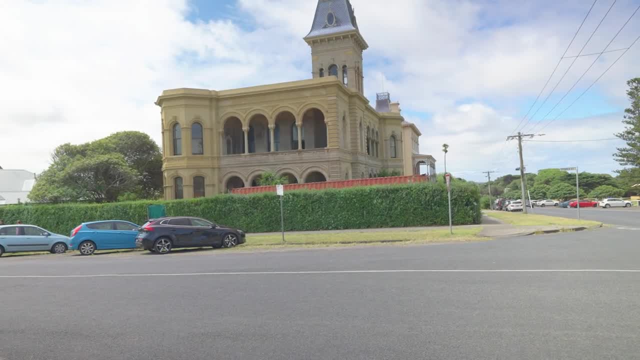 all of the masonry structures and we can see. it's quite beautiful with all its arches, acting in the way that masonry wants to act. Whether we're looking over the windows with the keystones or between the pillars, we can see if it's built and detailed correctly, it can lead to quite a 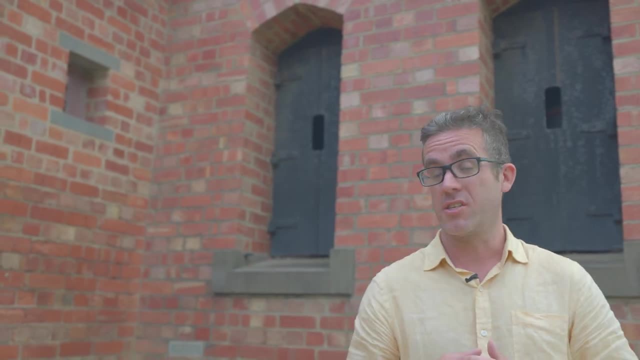 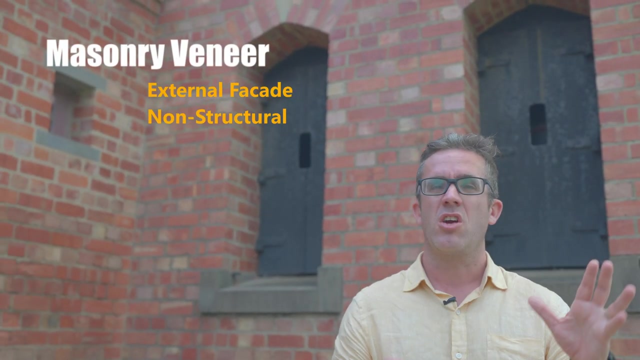 beautiful design. There's also a number of ways of how masonry structures can be built. Sometimes you can have it as a masonry vineyard, which is more our typical build. where you've got the masonry on the outside, It's only really acting as a cladding to the building, and then you'll either. 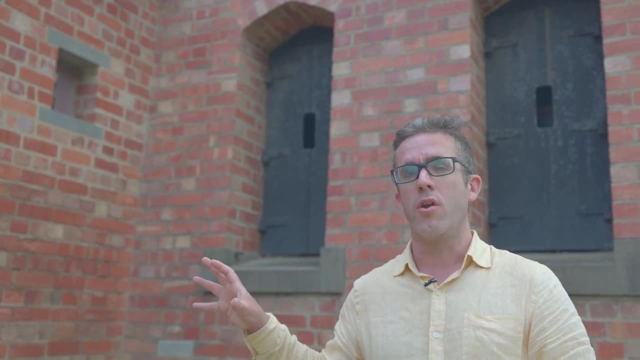 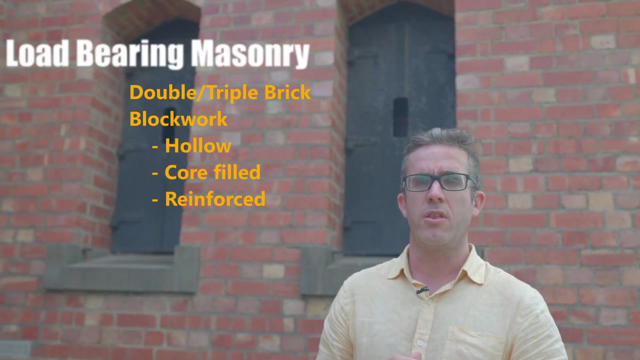 form up the main load-bearing element. or if we look at this fort, these walls are definitely load-bearing. This is a load-bearing masonry design where you need to be a little bit more careful with your design, as it will be taking vertical loads. Any good masonry design needs to. 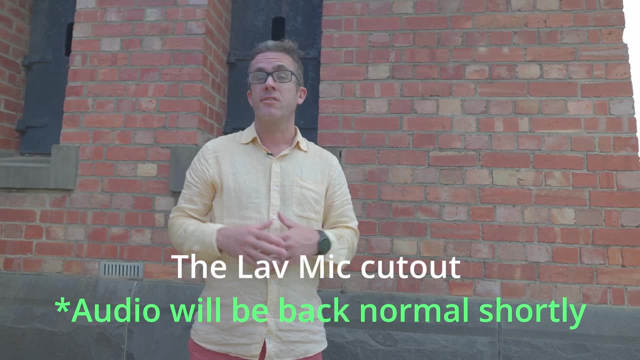 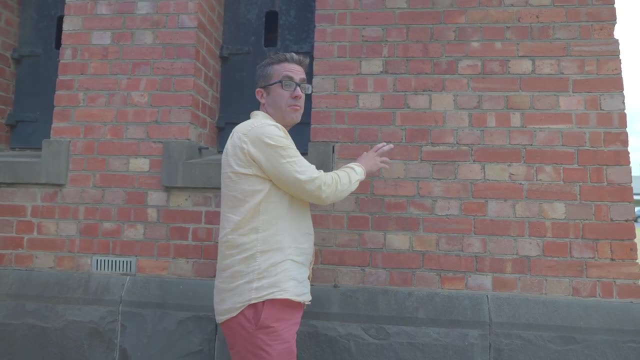 consider the dimensions of any brick, as if we need to cut bricks it's really wasteful to design. So if we look at our traditional brickwork that we can see here, we can really determine the dimensions of the bricks. So we've got a 230 long brick across here. it's 90 high. 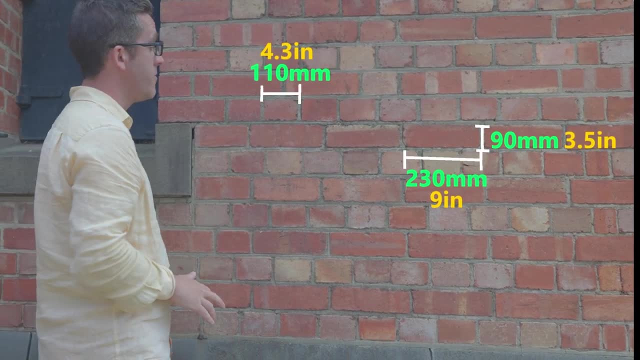 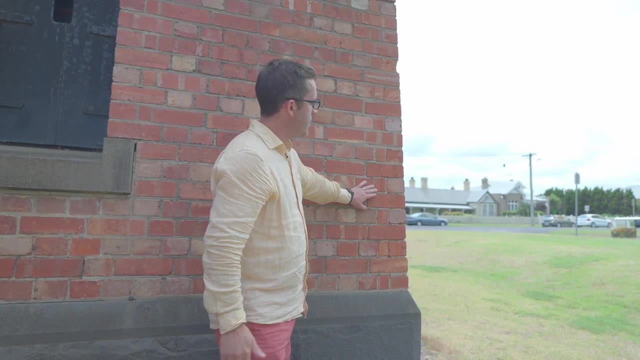 and it's one 10 thick. So we can see that from our brick here. the dimensions of the brick Now, if we move along, we can see that because of this building moving in it didn't quite line up so they had to cut several bricks to be able to lay out this brickwork. So this means there's a 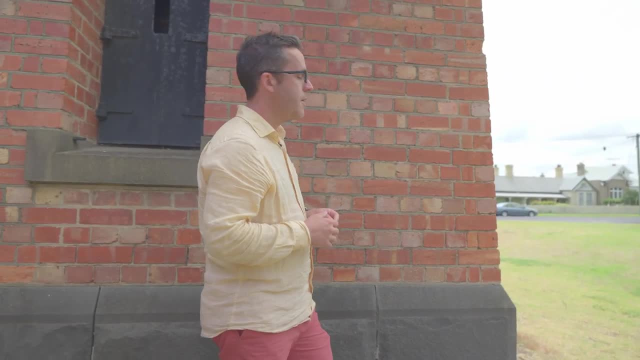 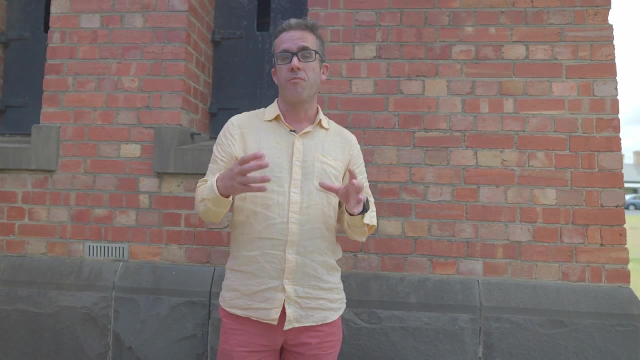 lot more work to cut the bricks where, if you had made it slightly smaller, they may not need to have done this, making it a more efficient design. Now, when you're designing masonry, there's also different dimensions of brickwork, So if you're doing concrete bricks, they will come with. 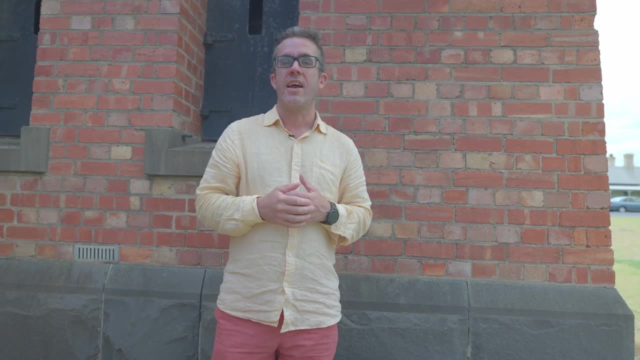 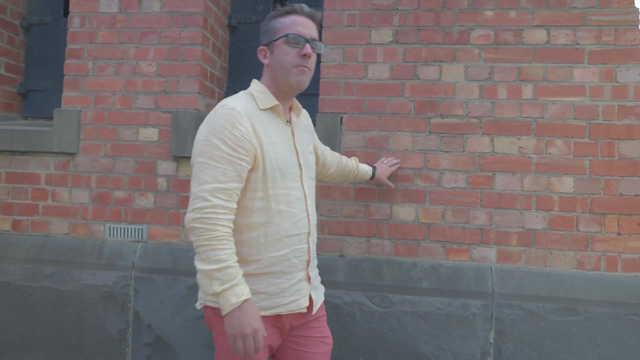 different dimensions And when you're trying to lay out the length of your wall, trying to maintain in those unit lengths, the construction of a brick wall is made up of a number of different segments. So we've got our traditional bricks here. Now, bricks also come in two different types, So we've got our clay bricks. 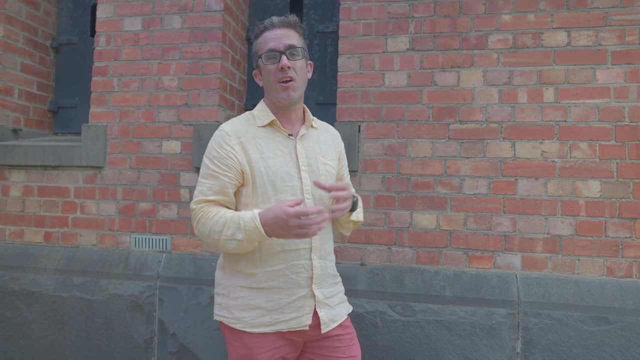 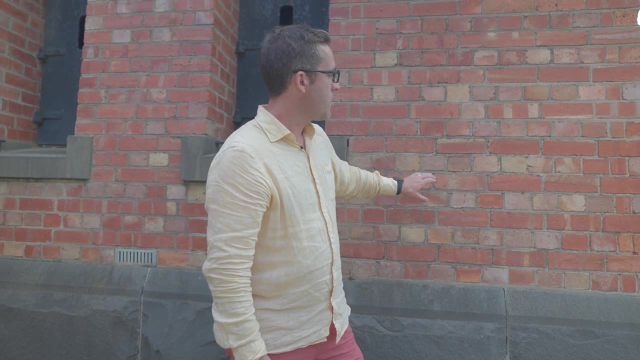 here, which is more of a common one, but they also come in concrete and they also have different properties. So you want to try and make sure you're not mismatching different types of brickwork. But if we're looking here, whether we're using clay or concrete, they still have a similar. 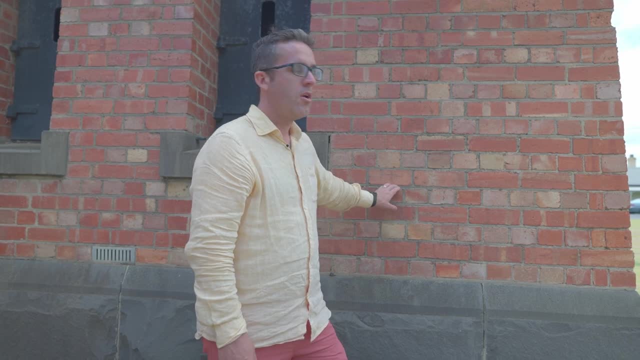 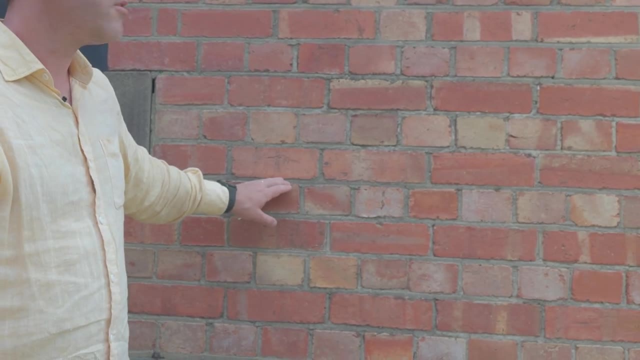 feature, as you've got your clay brick here and you also have your mortar. So building is built up of different elements. when you're doing your masonry design, You've got your brick, but you'll always have your mortar, So your mortar is essentially joining the bricks together to 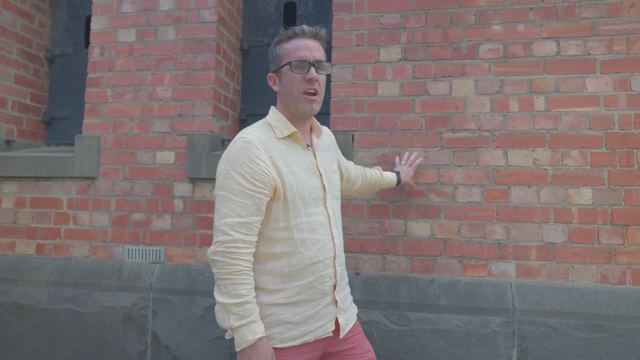 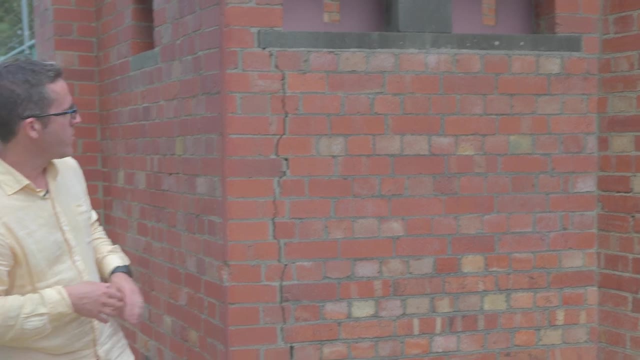 allowing for that interlock and making sure they're laying correctly. Not every brick is exactly the same, so you need to have some tolerance. Another key thing you need to worry about in masonry design is how bricks actually perform. One of the key elements is the failure of bricks is a brittle. 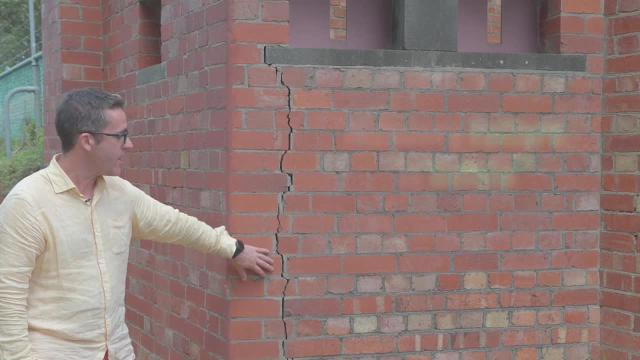 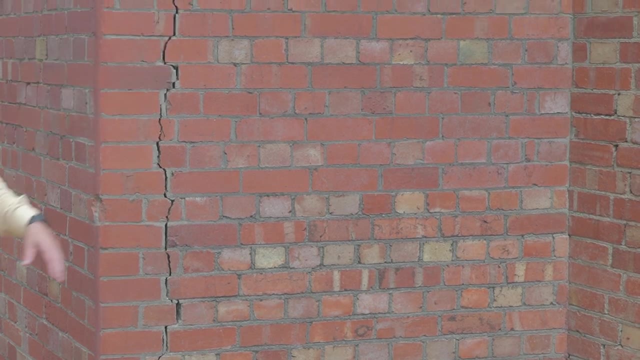 failure. So it's like a concrete structure without the reinforcement And we can see that through this joint here. So there's been somewhat restrained by the corner and the piers forcing a crack through this location. So you need to be carefully consider. 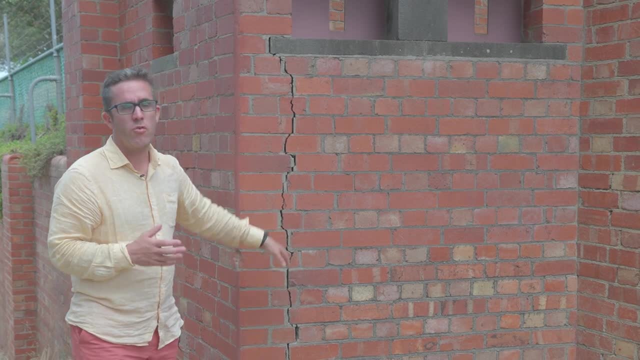 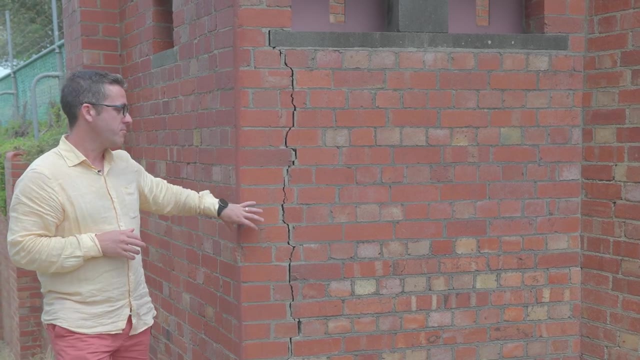 when detailing your structures, making sure you're not causing any of those restraints, or if you are putting in articulation joints. Another key thing about any masonry design, whether it's that block or that clay brick that we see here, is the fact that they're porous. 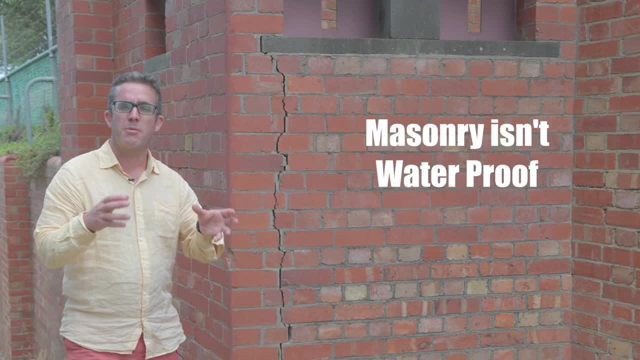 They'll allow water to flow through them. So on modern structures, you'll typically see a damp, coarse membrane at the bottom. They'll allow the water to flow out. But if you're building a masonry design, you're going to want to make sure that you don't have. 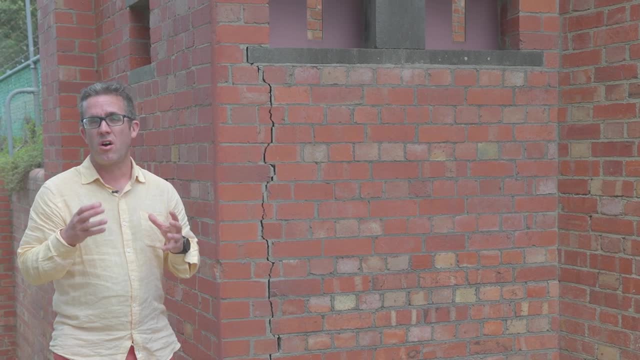 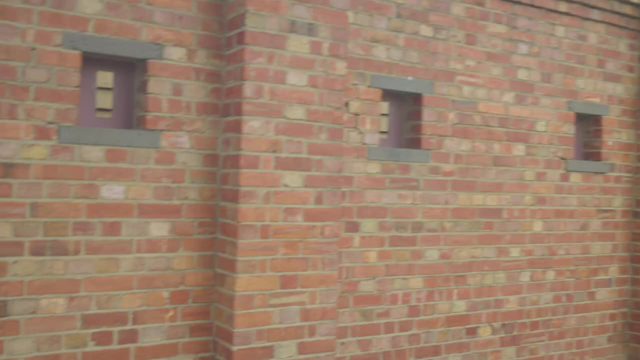 any timber or steel up against them, You need to make sure you designed it for that external use, So you either need to galvanize it to protect it for long-term or have the appropriate timber in these locations. Another key thing about any masonry design is the fact that you need to span.